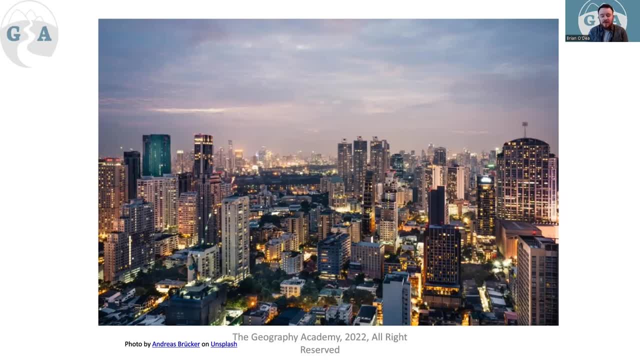 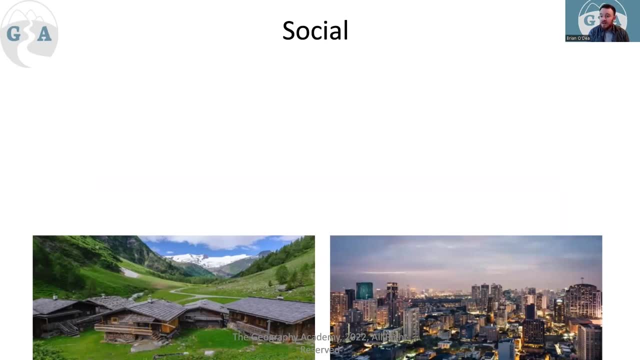 parks, lights and so on. We see a lot of high-rise buildings, lots of different transport facilities, very different and a harsh contrast to the other one. So this one would be densely populated here. So we divide most things up into S-E-E-P, so those could add the impacts of a volcanic eruption, think. 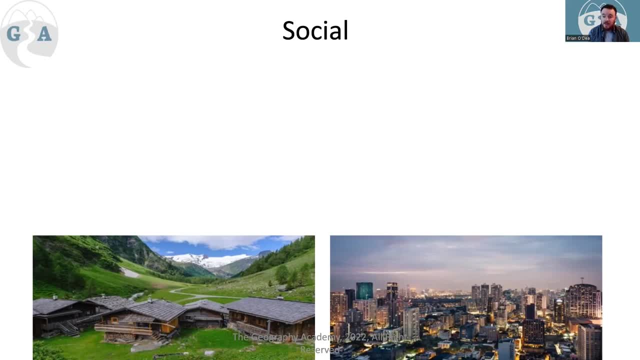 S-E-E-P: Social, economic, environmental and political. We divide it up into this because it allows students then to talk about different topics, so you don't get caught up talking about the same point, repeat yourself and it just makes you think a little bit more. Social reasons why. 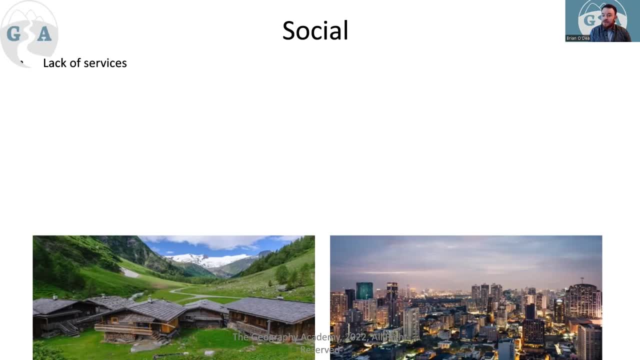 this is sparsely populated, Well, the one on the left is going to have a lack of services, so you're not going to have a lack of services. so you're not going to have a lack of services. so you're not going to have things like, let's say, hospitals. you're not going to have, maybe, sports grounds if 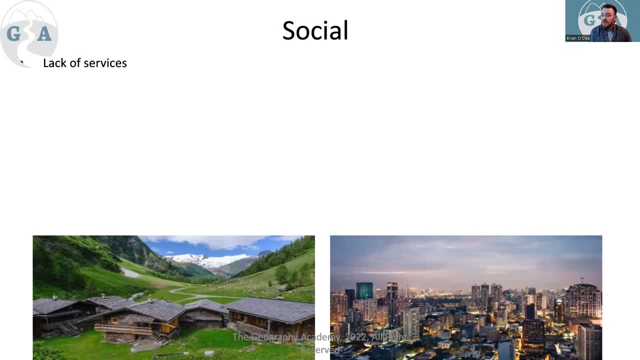 you like playing football or that type of thing. So yeah, you're going to be lacking some of the services there so people might not want to live there. Education, then, as one of the services: so different levels in different places, like a sparsely populated area, may have a primary school. 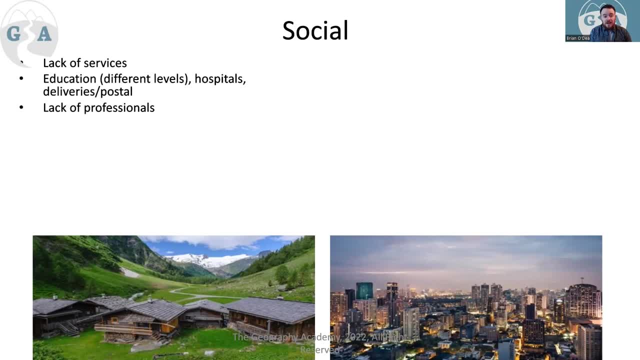 but it's unlikely to have like a secondary or high school level. See a lack of professionals, which means they can't offer the work anyways there like teachers, doctors, postal workers, Reduced amenities. things to do in the area might be limited For some people. they would look at a landscape like: 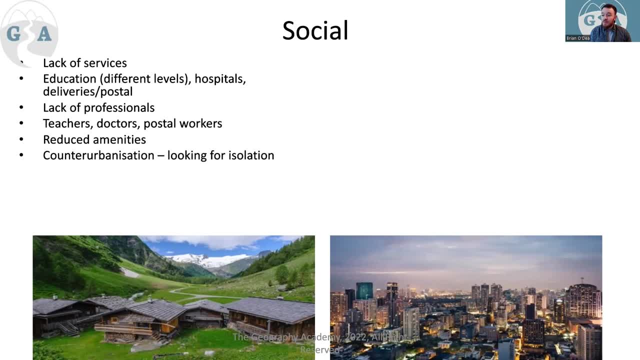 this and say, oh, this is lovely, there's lots of outdoor things to do. but for other people who don't like that, they might not find there's too much to do there. Counter-urbanization though, we might see changing the trend, so people might be looking for isolation and want to move into. 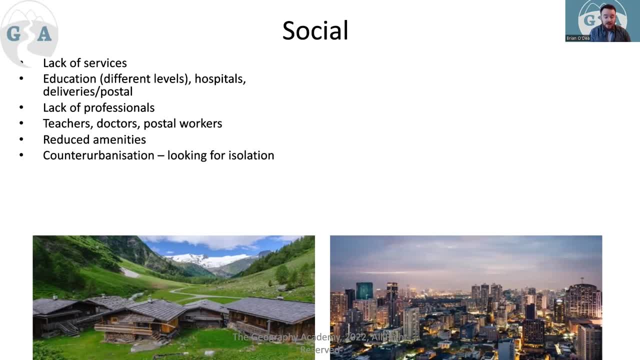 isolated communities where there is a sparse population, trying not to increase it too much and certainly not encouraging people to move around them. We look at mechanization of agriculture and mining, meaning there's not many jobs in the rural area now, so we see sparsely populated people. 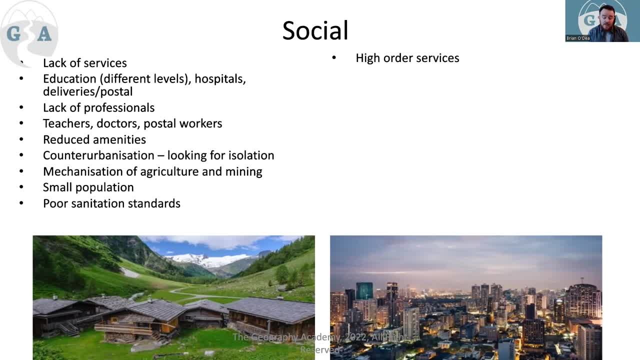 because they can't get jobs in the area High order services. then what does that mean? It just means, like we said on the left there, with education, so for them they might have things like a university and they might have specialist doctors for certain diseases, for instance, which might not be the case.